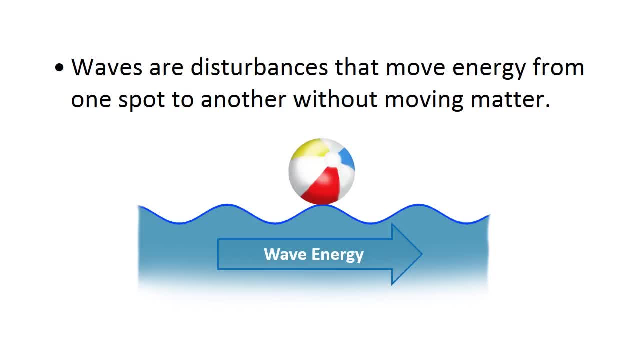 a river traveling in one direction. These are just energy waves traveling through the water. Another good example is: if you take a rope and you flick that rope, the energy will travel down the rope and you'll have a wave traveling down the rope, but pieces of the rope are 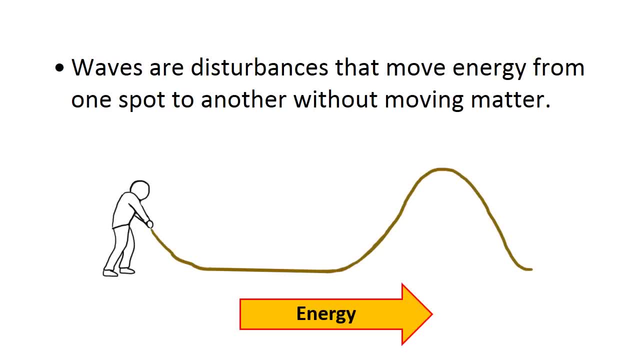 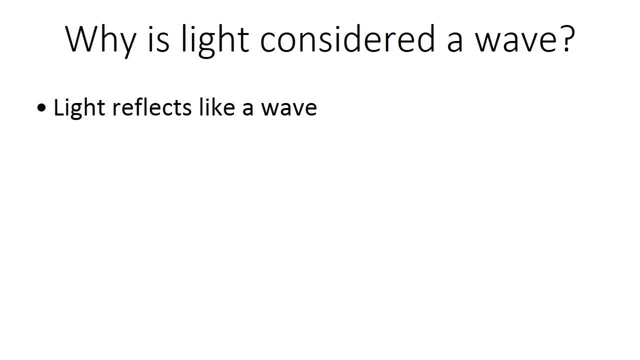 not actually physically moving down the rope right. The piece that was in that started in your hand is still in your hand at the end. So the disturbance of energy moves through the, the substance, but it's not moving matter As it goes. Now why is light considered a wave? There's several reasons. Light 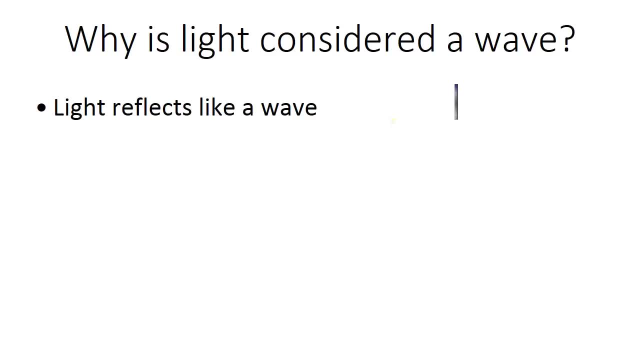 reflects like a wave, So we'll be talking about this in later videos. So light bounces off things. Light refracts like a wave, So when it goes through into a different medium it will bend and change direction and light will interact with itself to create interference patterns like a wave. So here's an example of the. 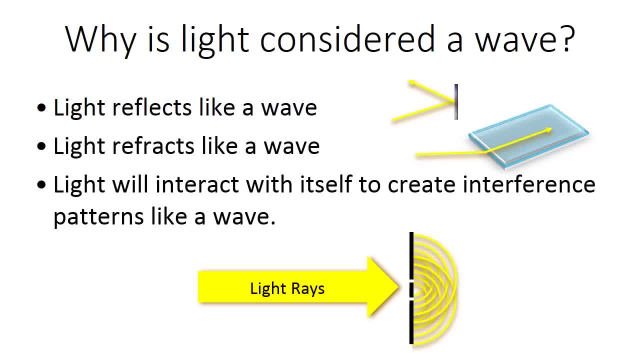 double slit experiment. Light rays pass through here and then it's like the waves sort of overlap and create giant crests and troughs and stuff. I'm not sure if we're ever going to talk about this, but there's some really good videos on YouTube. Just look at the. 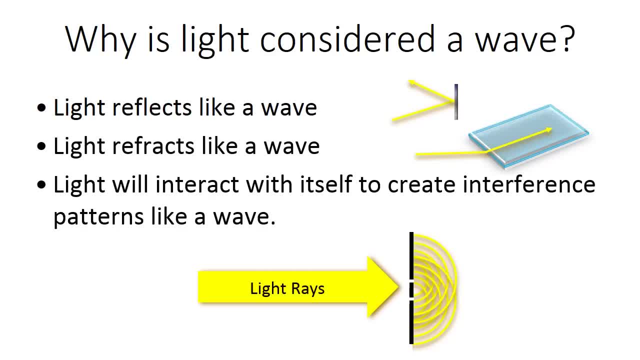 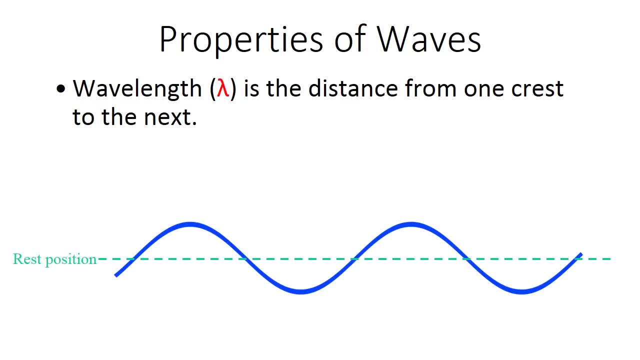 double slit experiment. Look that up and it explains it fairly well. So now we'll look at some properties of waves. First off we'll look at wavelength, and this is distance from one crest to the next crest. I guess it could also be from one. 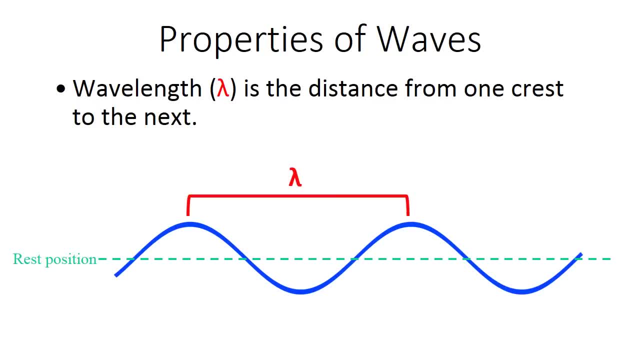 trough to the next trough, or really any one point on a wave to the same point on the next wave would be the wavelength. Amplitude is the waves height above the rest position. So it's not the height from the bottom of the trough, It's just. 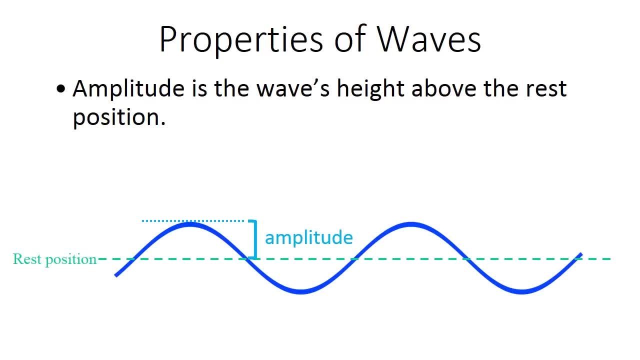 the height from the middle, the rest position. So if there's no waves, the water would be where that dashed line is. It wouldn't be way down in the trough. So that's the amplitude. The amplitude is also the depth below the rest position. 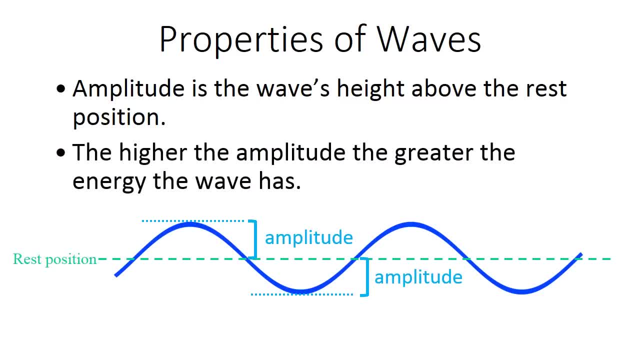 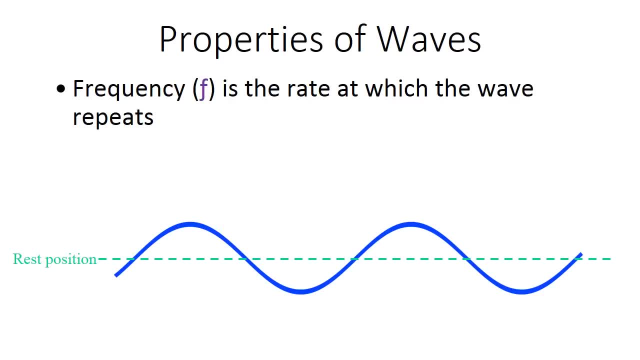 It'll be pretty much the same as the height above, And the higher the amplitude, the greater the energy the wave has. So the higher the waves, the more energy there is. Frequency is the rate at which the wave repeats itself. So frequency is measured in Hertz, and Hertz is the number of waves per second. So if we say 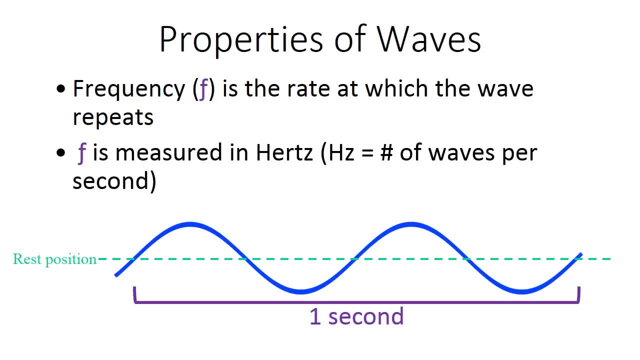 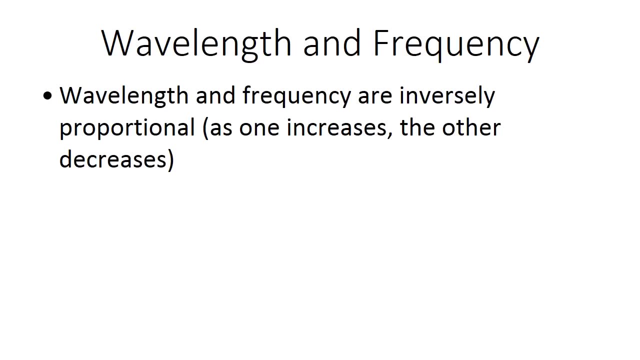 this is one second And we have what is that? one, two, We've got two crests or two full cycles of the wave there, So that's two Hertz Wavelength and frequency. Wavelength and frequency are inversely proportional, And that means as one increases the other. 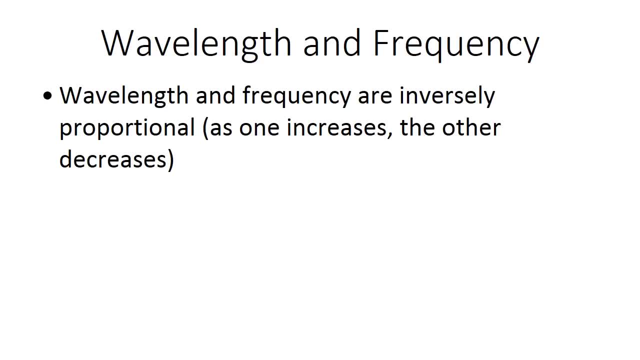 decreases. So if your waves are longer, obviously your frequency is going to go down. So as the as the waves get bigger, the frequency gets smaller. So the waves happen less often because the waves are longer. That makes sense. The speed of a wave v can be. 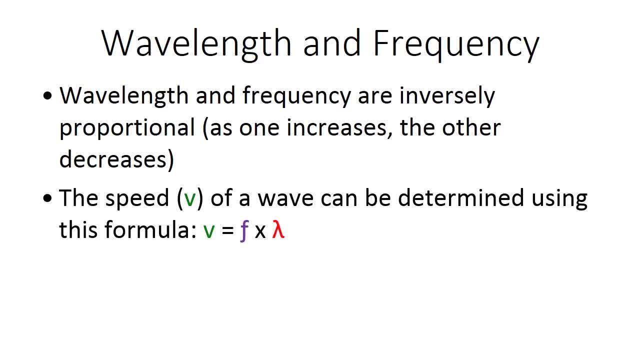 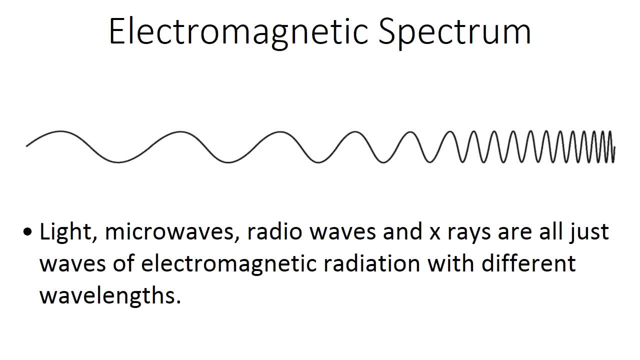 determined using this formula: V equals f times lambda, Or speed equals frequency times wavelength. So now we're going to look at the electromagnetic spectrum. Now. light, microwaves, radio waves, x-rays- these are all waves of electromagnetic radiation That have different wavelengths, So all these things are basically the same. 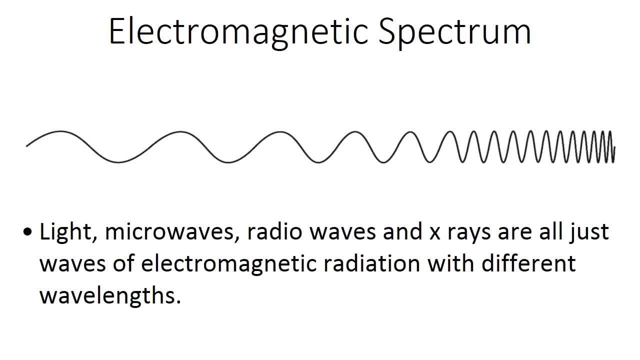 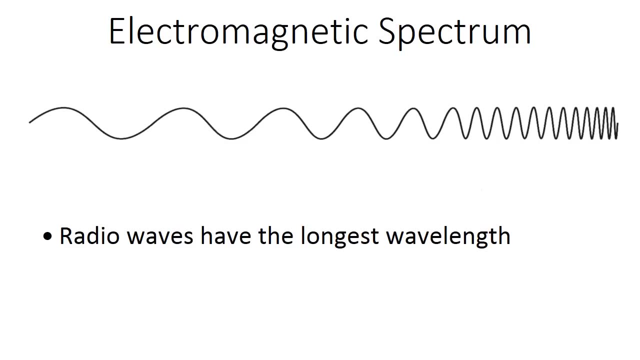 stuff. It's all electromagnetic radiation. The only thing that's different is the length of each wave of that electromagnetic radiation, And we use it differently. So we're just going to go through a couple different categories of electromagnetic radiation and what we use it for. We'll start off with radio waves. 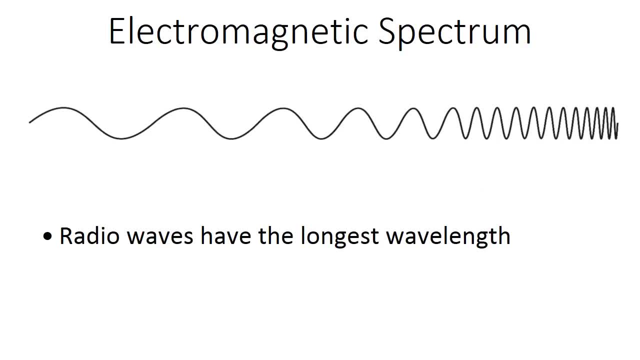 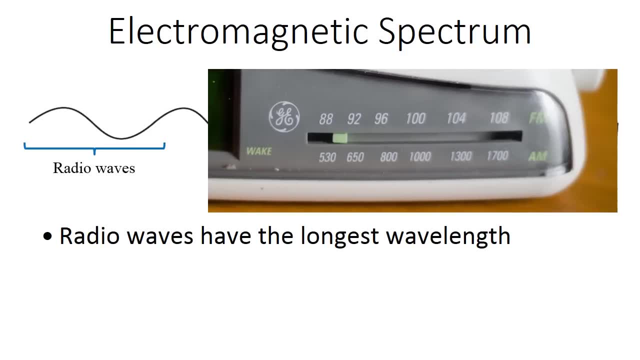 which have the longest wavelength out of the ones that we're looking at And they're going to be way over here at the left. So we're going to go to the left side where the wavelengths are nice and long. If you look at any radio, those numbers, there are the frequencies you're tuning. 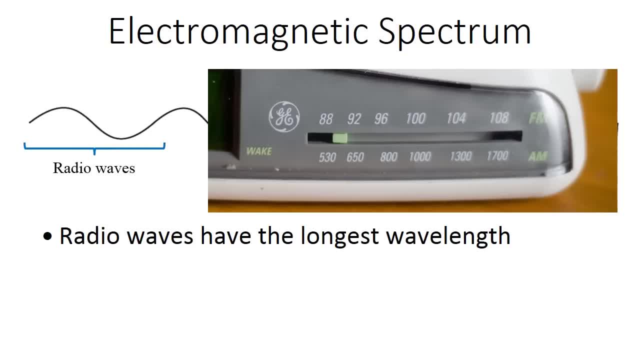 into And I think I'm at around 89 here. That's the channel I'm on, So at that frequency the wavelength is actually around three meters. So if you've ever been driving in a car and the radio is not coming in clearly and you can drive. 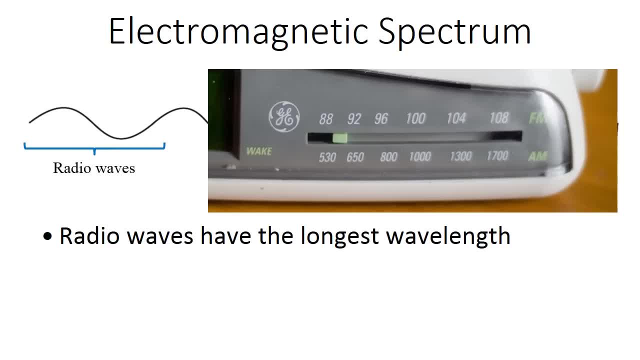 a little bit further up. you know, just drive your car up a meter, it starts coming in clear. That's because you're hitting another crest of the wave, of the radio waves that are coming off the radio antenna, wherever that is After. 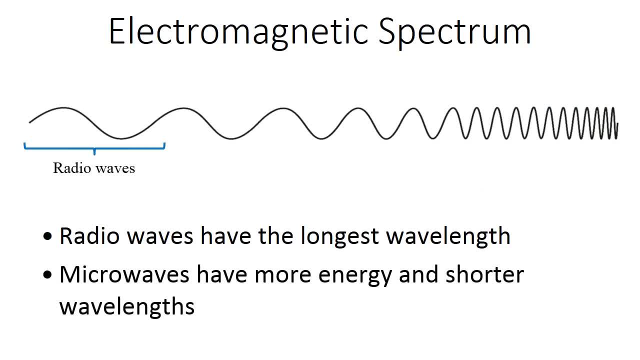 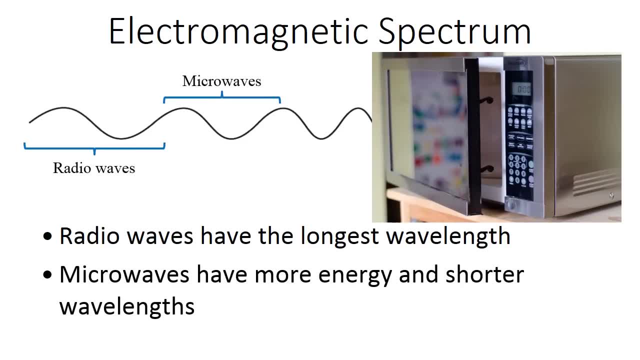 radio waves, we have microwaves. Microwaves have more energy and shorter wavelengths than radio waves, So they're the next ones there And we all know what microwaves do. They heat up our food And they don't heat up their food because 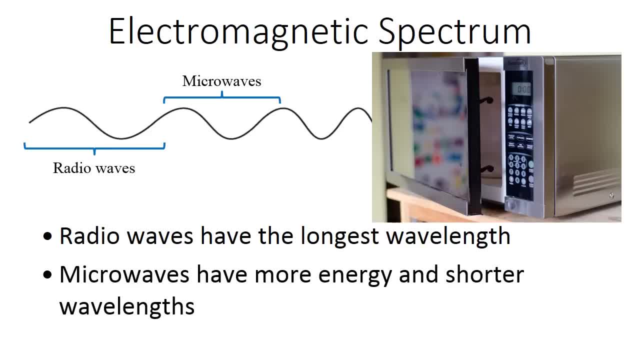 microwaves themselves are hot, It's because they cause all the atoms in something to like in the food, the egg or potato or whatever it is, to start shaking around a lot. But microwaves do have more energy than radio waves, So 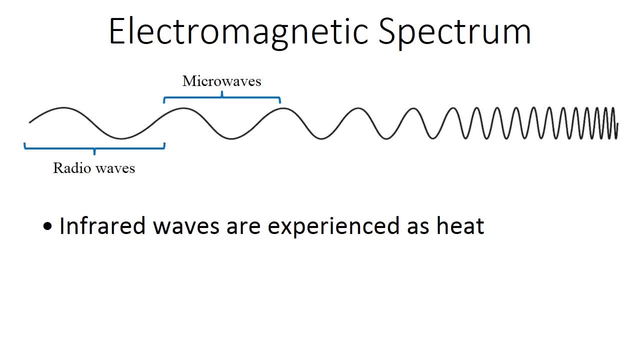 after microwaves we have infrared waves And these are often experienced as heat. So the radiation that comes off of a stove- if you're standing near a stove or off a radiator in your home, would be giving off infrared radiation, And these are found basically just up from microwaves And, interestingly, some. 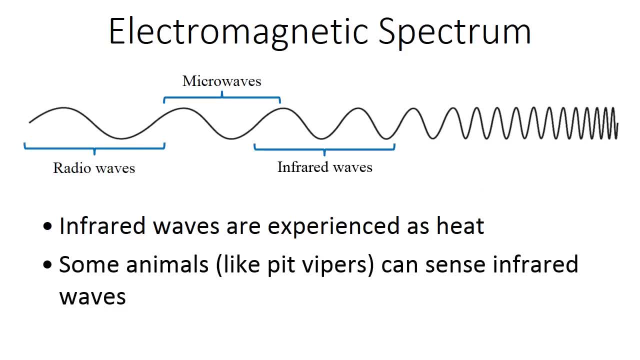 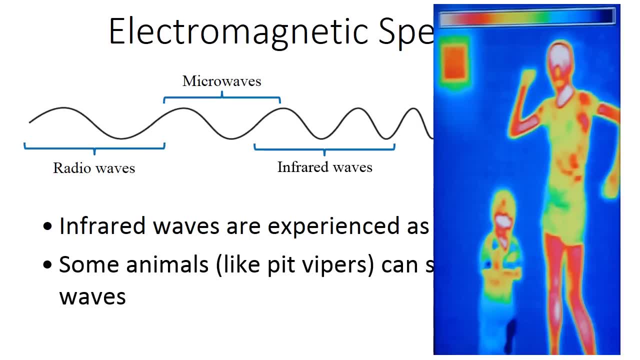 animals like pit vipers, such as a rattlesnake, can sense infrared waves. So if a rattlesnake was looking at you, it might see something like this if you were dancing weird beside a toddler. But those are infrared waves. This is a. 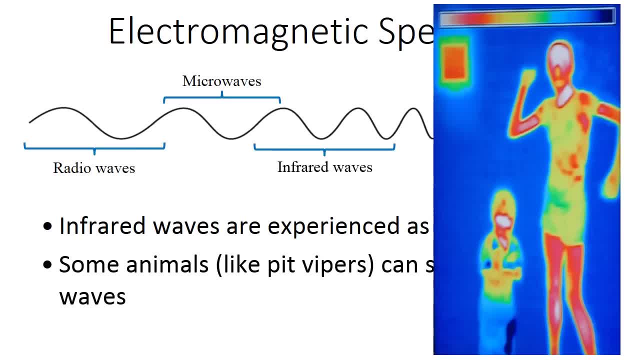 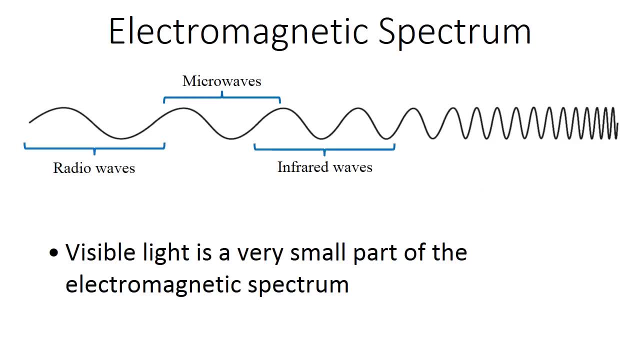 camera that's been set up to sense infrared radiation, So you can see the different levels of heat coming off of people. Alright, after infrared we have visible light. So visible light is actually just a tiny little bit of the electromagnetic spectrum, And in that, 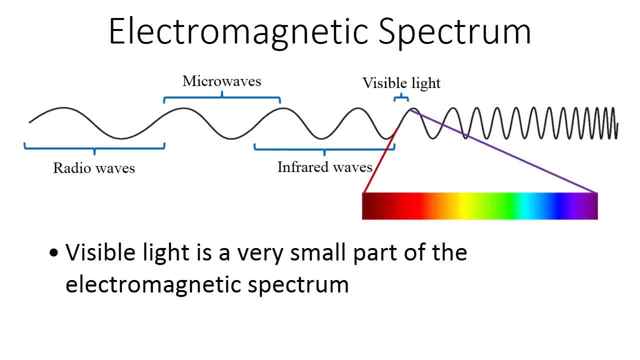 tiny little bit. we've got all the colors. We've got red, orange, yellow, green, blue, violet, all that stuff, But it's actually a very small part of the spectrum that we can see. After visible light we have UV light, And UV light has more energy. 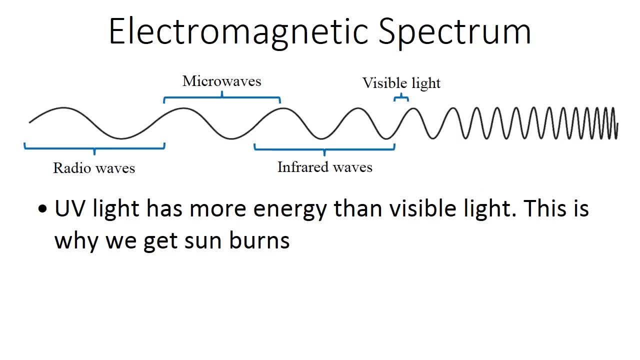 than visible light, which is why we get sunburns from UV light. You don't get UV light from lights in your house because they don't give off a lot of UV light, Whereas the Sun does give off UV radiation. so you get sunburns there. So the ultraviolet waves 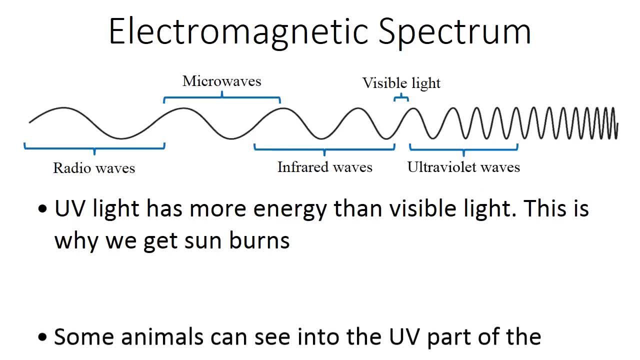 are past visible light, And what blows my mind is that some animals can see into the ultraviolet part of the spectrum. Now, if you think about it, what that means is that after violet they have other colors. So animals such as this guy, the American kestrel, can see into the ultraviolet range, Which. 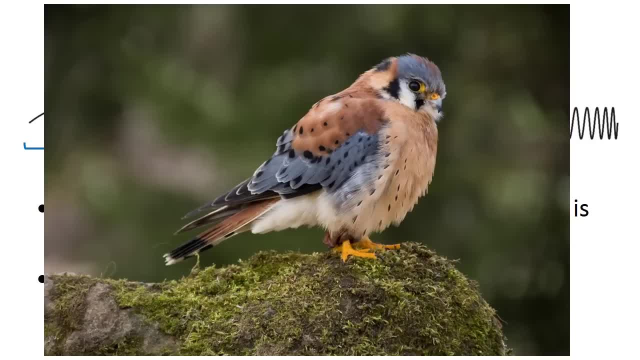 means that it can see more colors than we can, So its color wheel will have an extra color or two, And we can't really describe those colors because we have no concept of what they would be like. right Describing those colors to us would be. 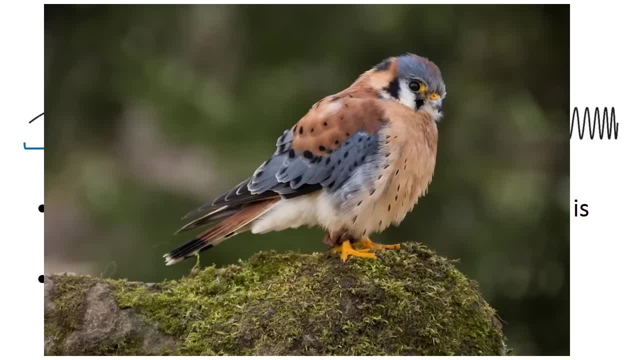 like describing red to a person that can't see it. We can't see red, So these animals can actually see other colors. I think there's other animals too. I believe bees can see into ultraviolet as well, And you may have seen artists renderings of what it might look like, but realistically, 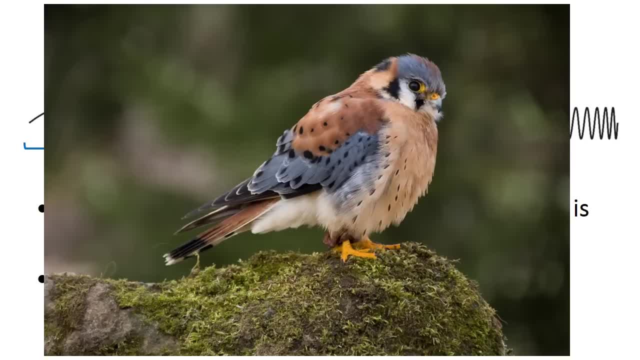 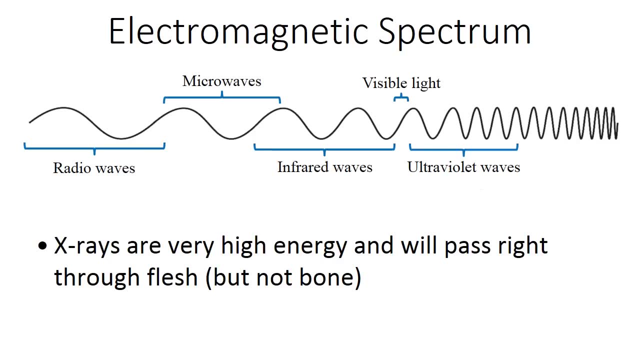 they can't show us what the colors are that these animals can see, because we are unable to see them. Alright, after ultraviolet we have x-rays. These are very high energy and will pass right through flesh but not bone, Which is what makes them helpful in medicine, because we can take x-rays of 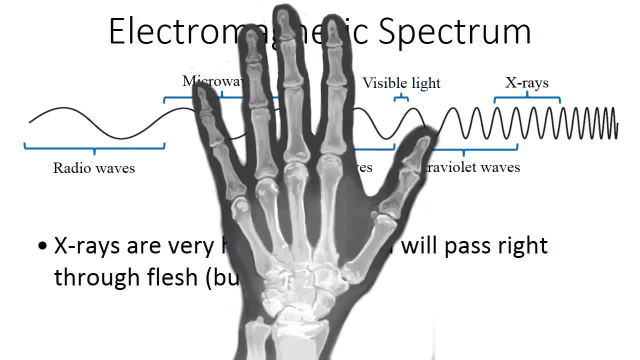 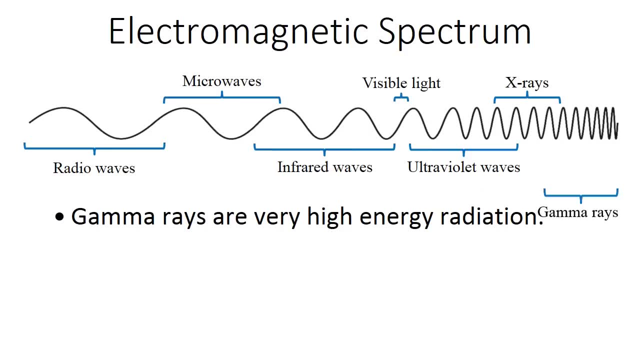 things and we can see what the bones look like, but they'll pass right through the rest of your, your fleshy bits. And last but not least, we've got gamma rays. Gamma rays are extremely high energy radiation. You don't want to get exposed. 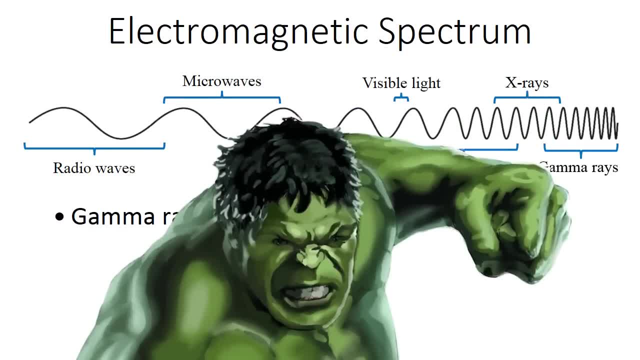 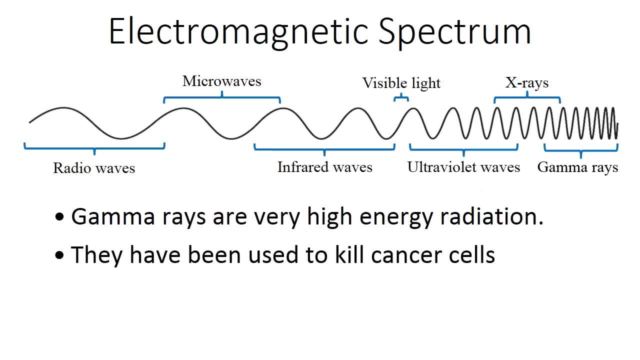 to gamma rays, otherwise you'll turn into this guy. Actually, no, you won't. you probably just get cancer. Gamma rays have been used to kill cancer cells. paradoxically, and gamma rays are produced by black holes and neutron stars, So it's very powerful radiation. 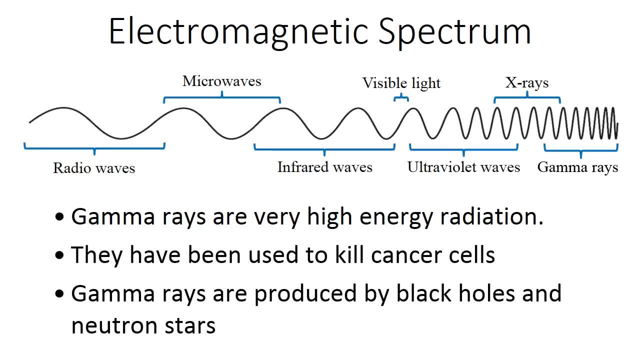 very high energy radiation. It's not produced a lot on Earth and I think a lot of it gets filtered out by our atmosphere. so you don't really run into gamma radiation a lot on Earth. But stay away from black holes because they're 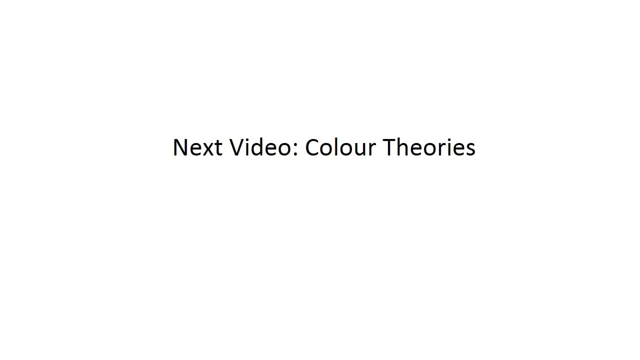 dangerous. Alright, so that's it for this video. Tune in to the next video on color theories. Thanks for watching.